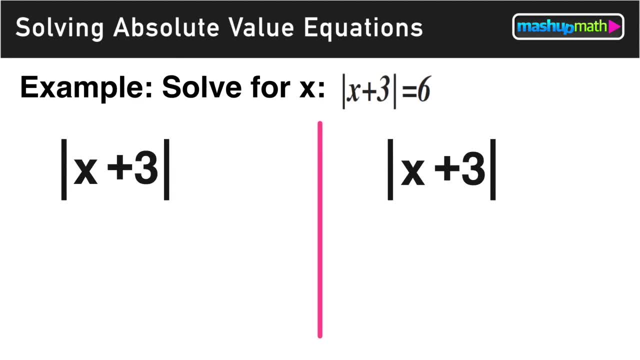 to solve for it twice, except that we are not going to include the absolute value bars. Now, the first equation we set equal to the value in positive form, and the second equation to that value, in this case 6, in negative form. So we're solving it for the 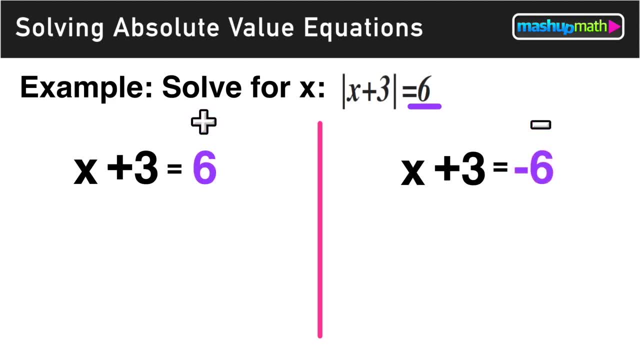 positive value and for its negative counterpart. So here we have, on the left side we're solving for the equation x plus 3 equals positive 6, and on the right side equation x plus 3 equals negative 6.. Now these are simple equations to solve. We'll go ahead and subtract 3 on both sides of the equal. 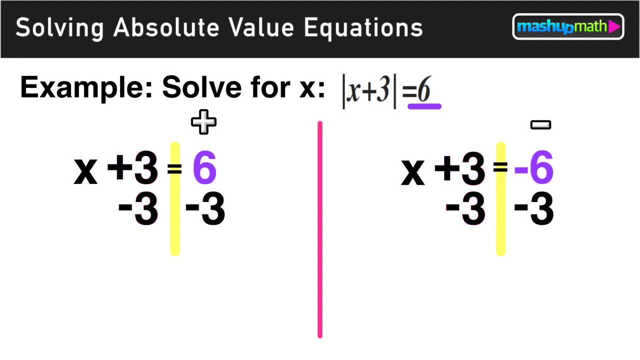 sign for both equations That will cancel out the positive 3 on each side. And now over on the right side of the left equation 6 minus 3 is equal to positive 3.. Over on the right side, equation negative 6 minus 3 is equal to. 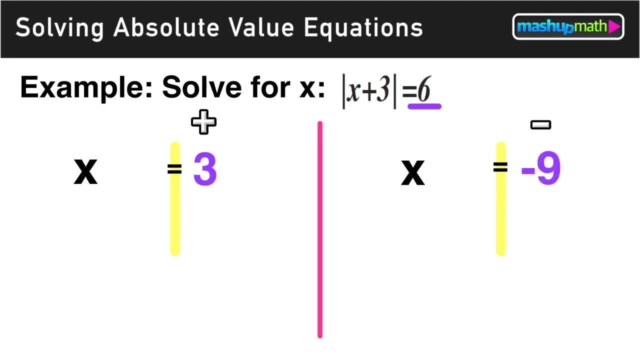 negative 9.. And now we have our two solutions to this absolute value equation: x equals 3 and x equals negative 9.. Now, to make sure that these solutions are correct, we can go ahead and do a check. So I take the original absolute value equation and substitute back in our 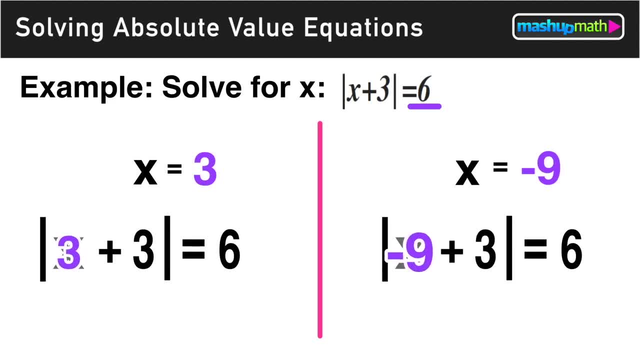 values for x. So on the left side equation I replace x with 3.. On the right side equation, I replace x with negative 9.. Now over on the left side, inside the absolute value, bars 3 plus 3 is equal to 6.. Over on the right side, on the absolute 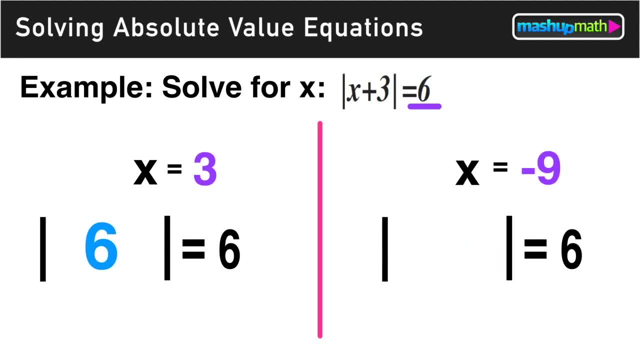 value bars. negative 9 plus 3 is equal to negative 6.. I know that my left side equation is true because the absolute value of 6 does equal 6, and I know that my right side equation is true since the absolute value of negative 6 also equals positive 6, so my 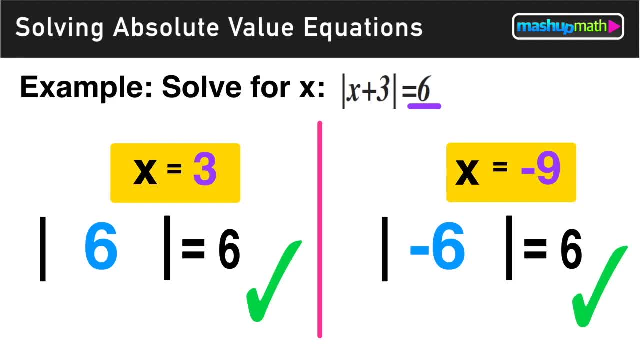 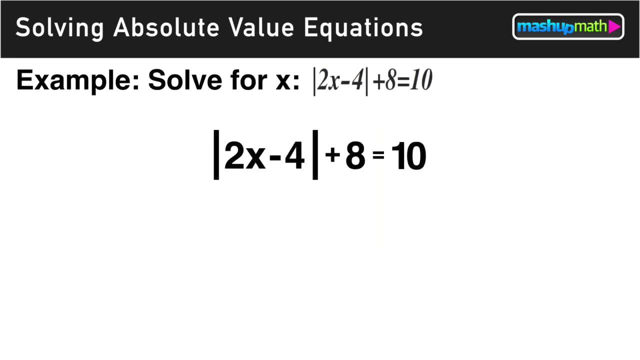 solutions of x equals 3 and negative 9. both check out. So now let's go ahead and take a look at another example. In this case we have the absolute value of 2x minus 4 plus 8 is equal to 10.. Notice on the left side of the equation that 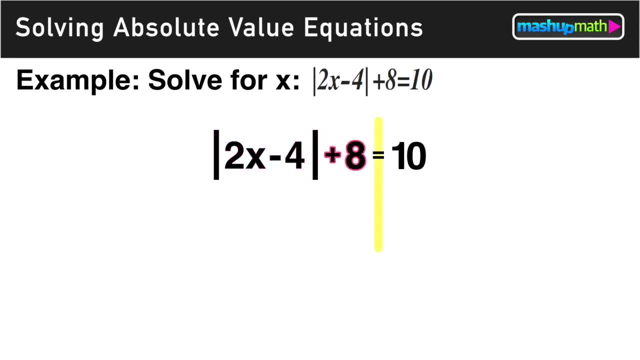 we have the absolute value piece and we have that plus 8.. Now that plus 8, we have to move to the other side before we can solve this. so lets go ahead and subtract 8 on both sides of the equal sign. that'll cancel out on the left side and on the right side, 10.